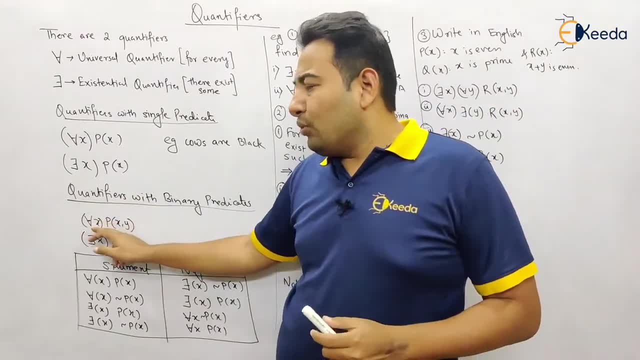 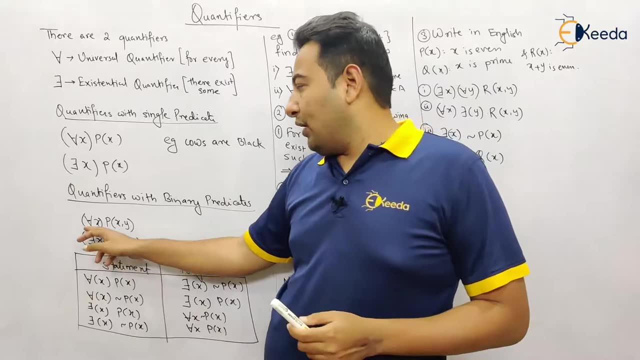 So there is a difference. Don't worry, It's again very simple. How to read this statement for every x. Now, this time it will become for every x. How to read this statement for every x: p of x- y is true. There exists some x for which p of x- y is true, So this is how we're going to read this. 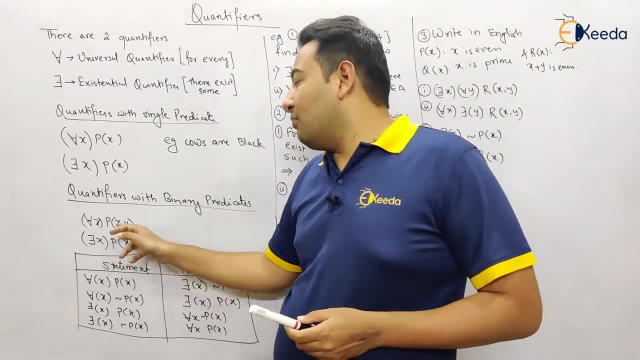 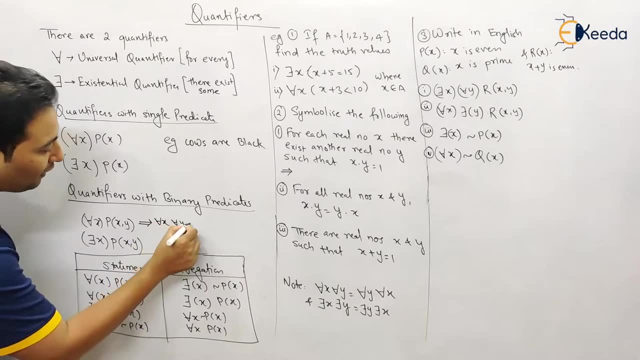 statement for every x- p of x, y is true. Now here the restriction can be on x and y, both on both. For example, see. this statement can be written like this also for every x. for every y, p of x. 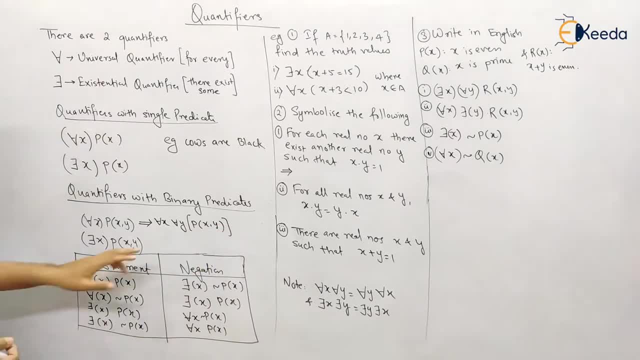 y is true. So restriction can be on both, Restriction can be on anyone, So choice is ours. For every x? p of x? y is true. For every x. for every y p of x? y is true, or it can be. 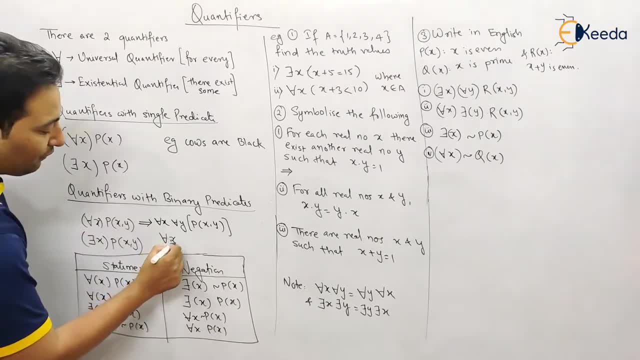 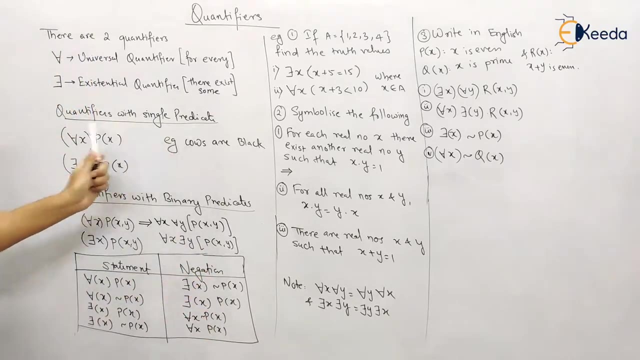 combination of universal and existential quantifier. let's say, for every x there exists some y, p of x, comma y is true, so there are number of possibilities. so that depends upon the problem here. binary predicates means there will be two predicates, x and y, and single predicate means 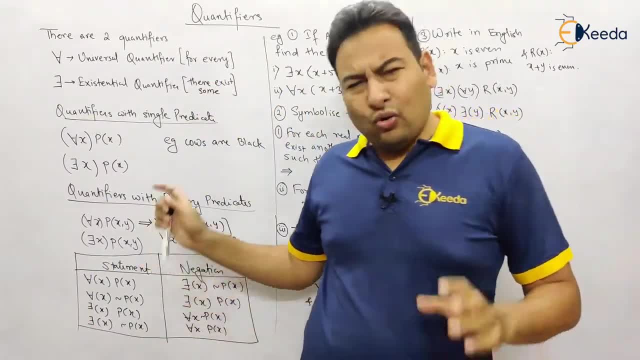 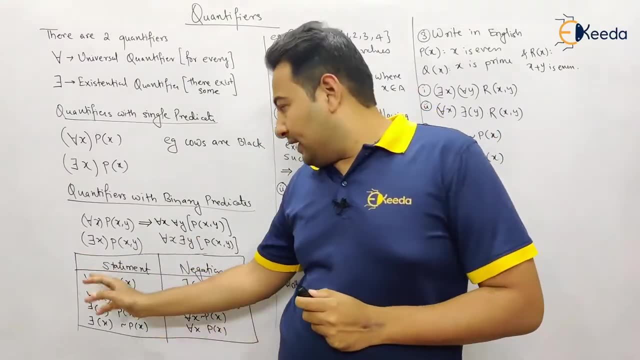 there will be only one predicate. let's talk about negation of a quantifier. don't worry with the example. all these things will be very clear. let's talk about the negation. see here: for every x px. suppose this is the statement that means for every x px is true, its negation will be. 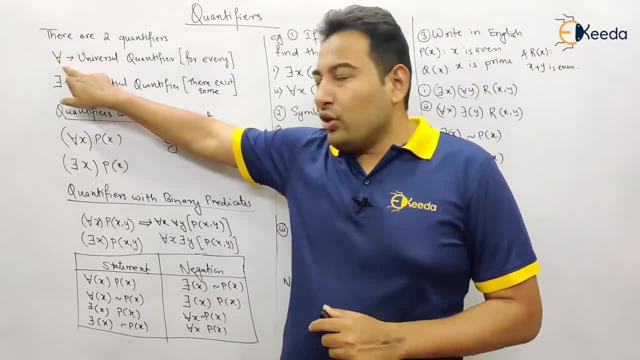 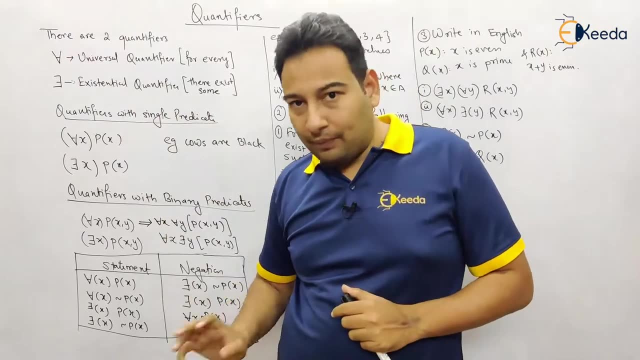 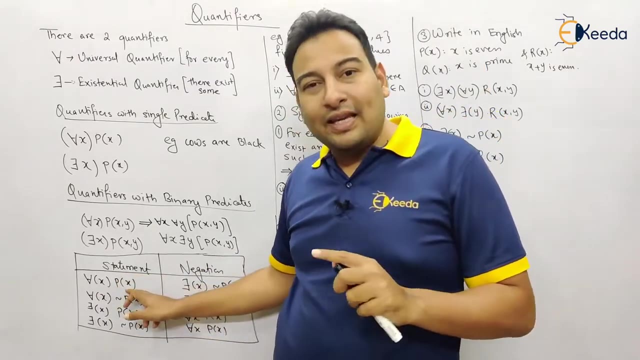 see, remember, universal quantifier: negation will be existential quantifier and existential quantifier negation will be universal quantifier. so if i have to take its negation, this is your universal quantifier that will become existential quantifier, and this is px is negation will be. 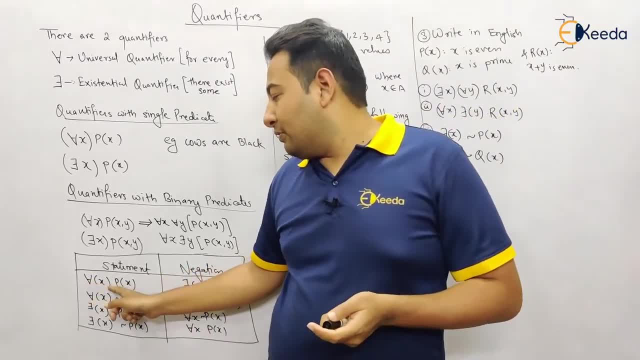 negation of px. that means for every x px is true will become a negation of px. that means for every x px is true will become a negation of px. that means for every x px is true. there exists some x px is not true, so this is the negation. there are four. 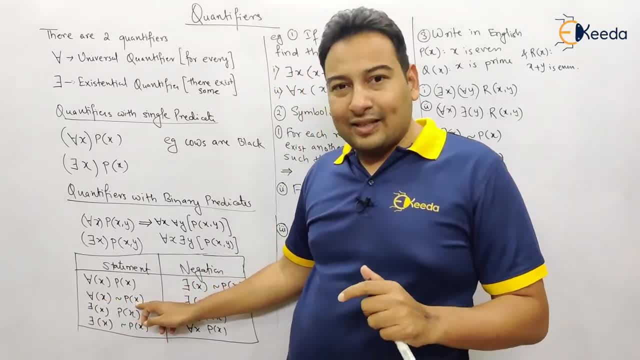 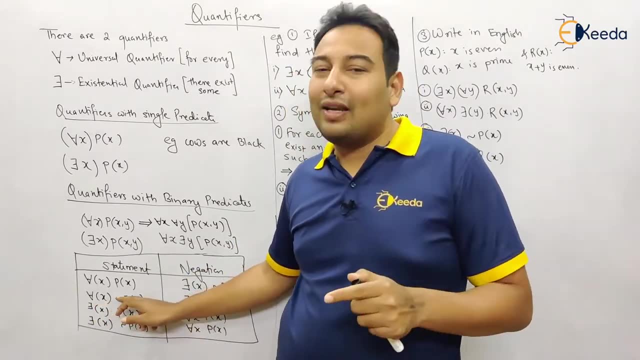 possibilities for every x, negation of px. again, it's very simple. if i'll take negation of the statement, for every will become there exist and negation of px. so negation, negation will cancel and get px. so there exists some x for which px is true. so if you want to read this statement, this: 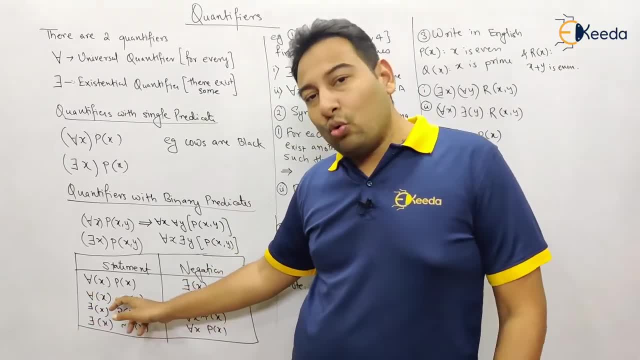 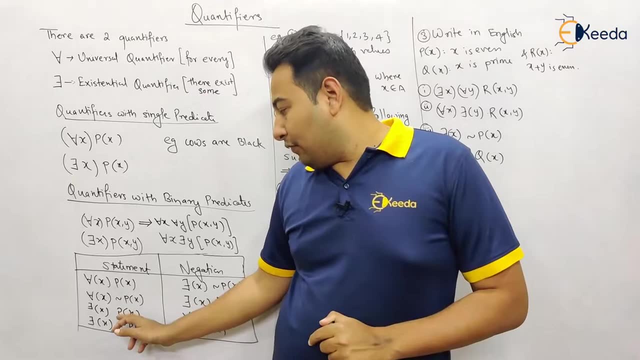 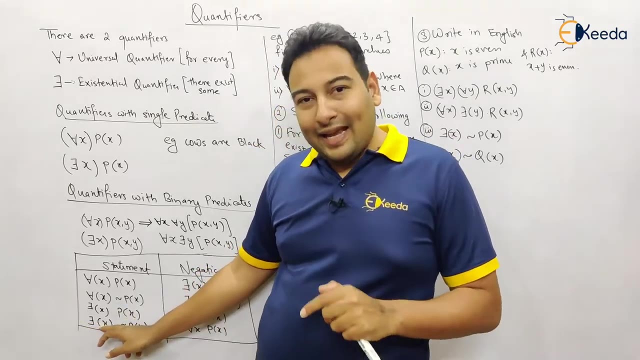 will be. for every x, px is not true. and if i take its negation, there exists some x for which px is true. there exists some x for which px is true. if you take negation, for every x, px is not true. and finally, for every x, there exists some x. if you take negation for every x here, px is not true. its. 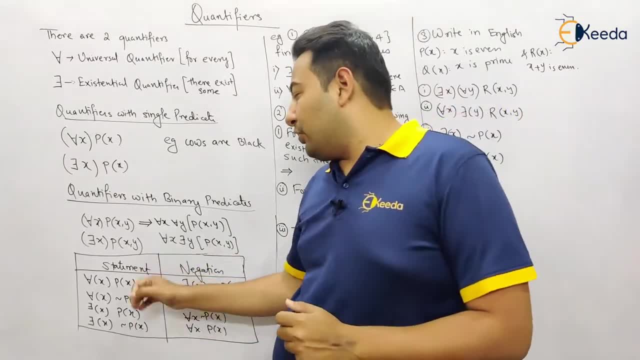 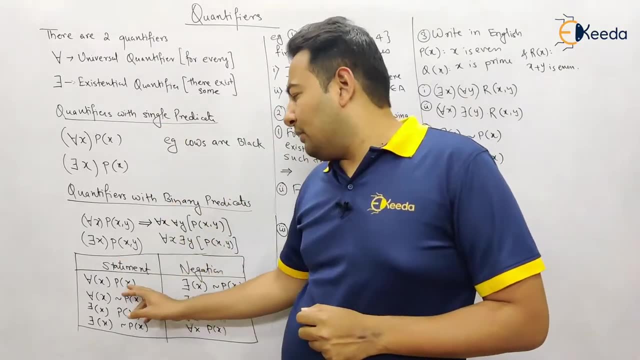 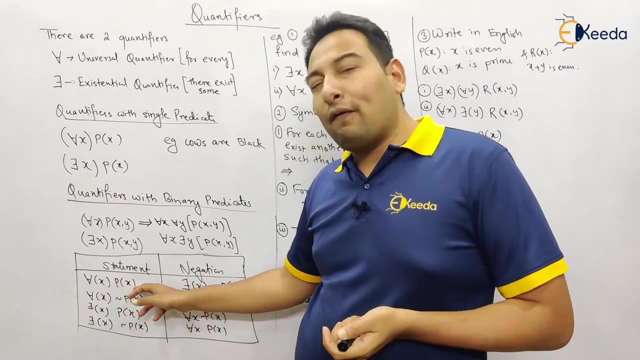 negation will become px is true. so these are the four possibilities that you need to consider. writing on the negation and obviously these negations are valid on binary predicates also. that means there can be two predicates also. for example, the same statement. it can be for every x, p of x comma y is true. if you take negation, that will become. 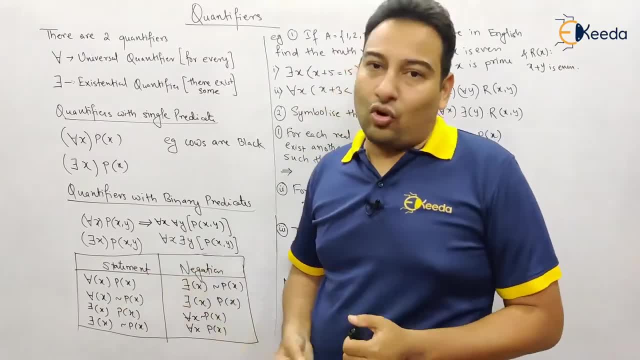 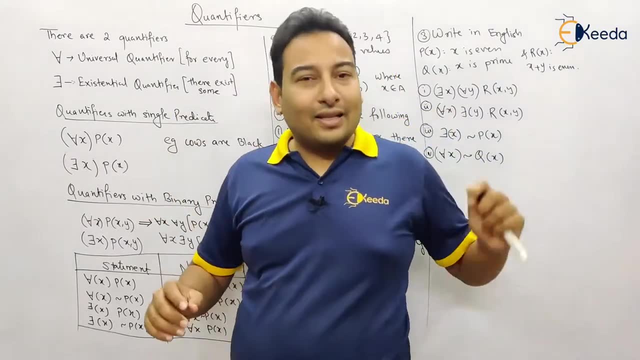 there exists some x for which p of x comma, y is not true. so this is what the concept is, what the quantifier is, how to read the quantifier and how to negate it. now we'll discuss with the help of example, and this will be very clear. it's a very simple topic. so let us discuss the first example. 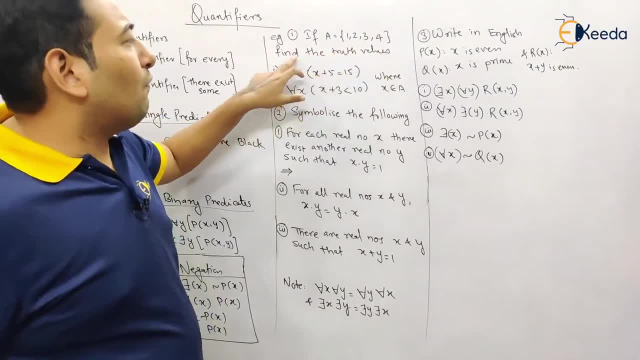 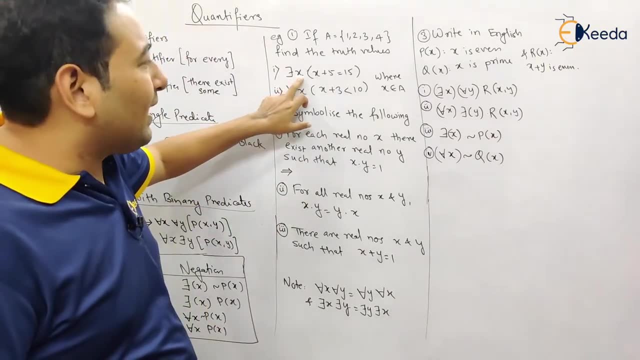 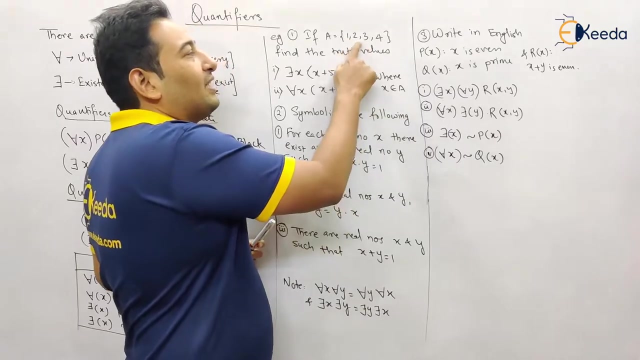 if a is equal to one, two, three, four, find the truth value of. we need to check whether this statement is true or false. see what the statement says. there exists some x such that x plus five is equal to fifteen. and what is x? x belongs to a. that means x belongs to this particular set. there exists some x for which x plus five. 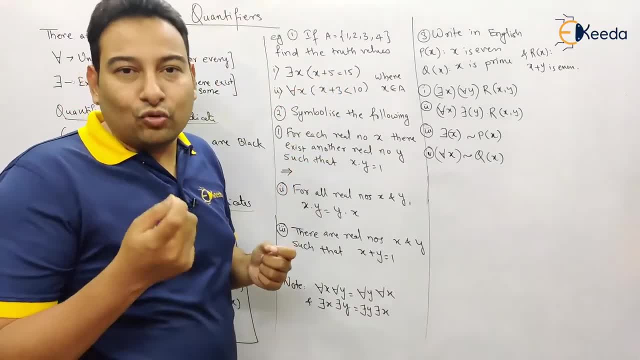 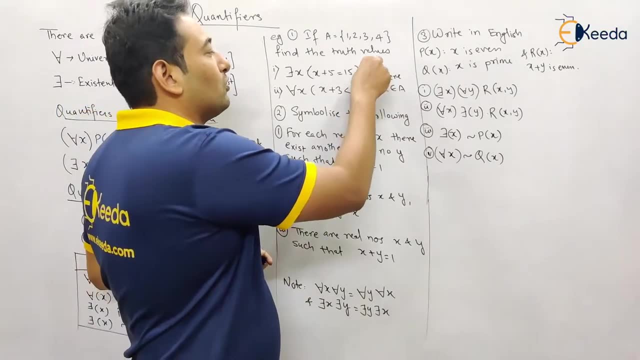 is equal to fifteen. now what should be the value of x? x has to be ten, so that ten plus five will become fifteen. but ten belongs to this set. no, that means this statement is false. is this clear? let's talk about the next: for every x, x plus three less than ten, so that's. 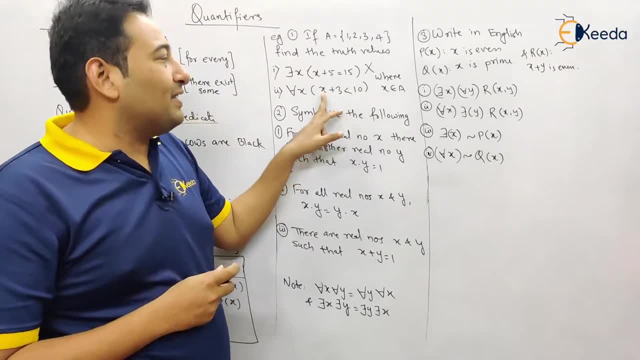 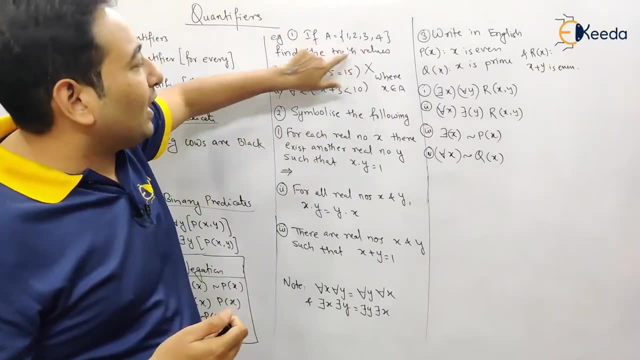 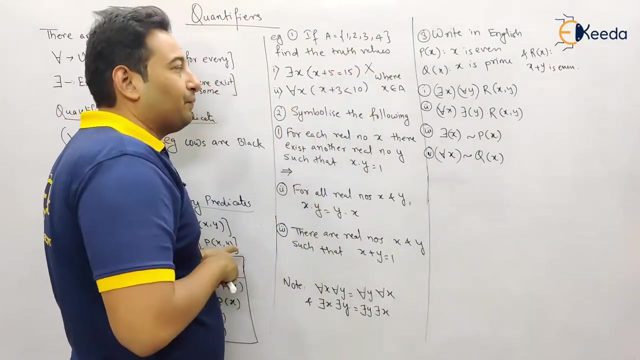 x plus three less than ten means x can be up to six, because six plus three will be less than ten. and if you observe this particular set, you put any value- one, two, three or four- the result will be less than ten. therefore, for every x, that means for all the values of x. this statement is true. 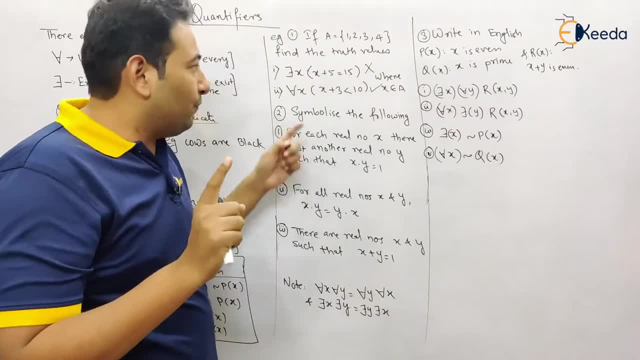 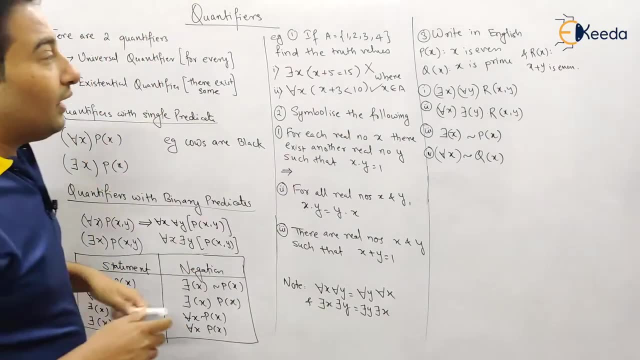 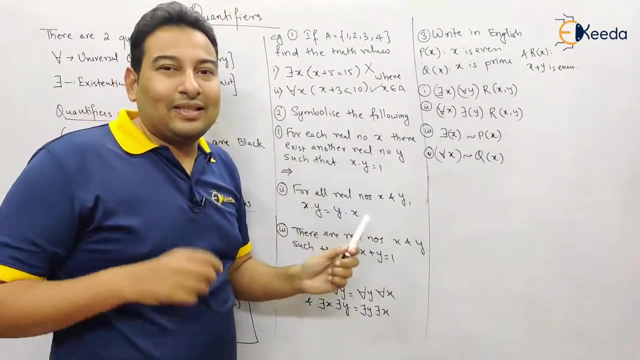 here there exists some x means x will be only one value here for every x means x will take all the values. this statement is true. next question now. this problem is based on the single predicate because there was only one condition on x. now, if you observe this example, this is binary predicate because the restriction is on x and y, both the 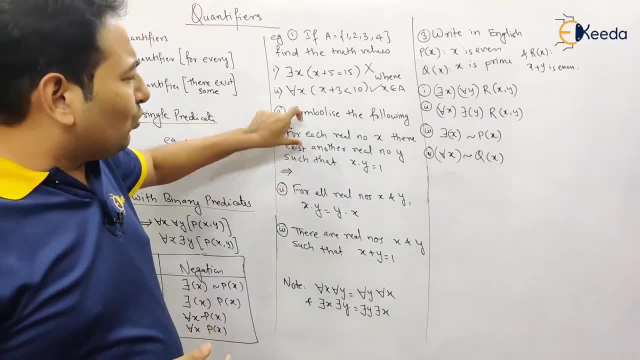 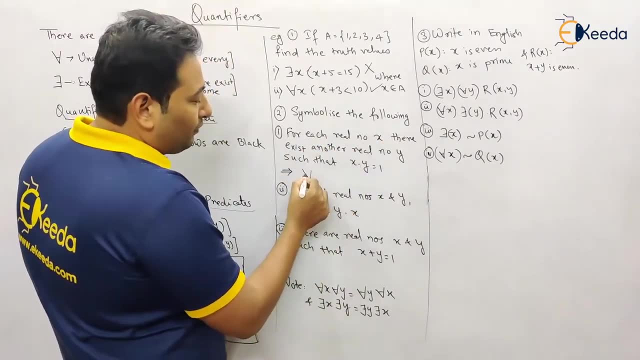 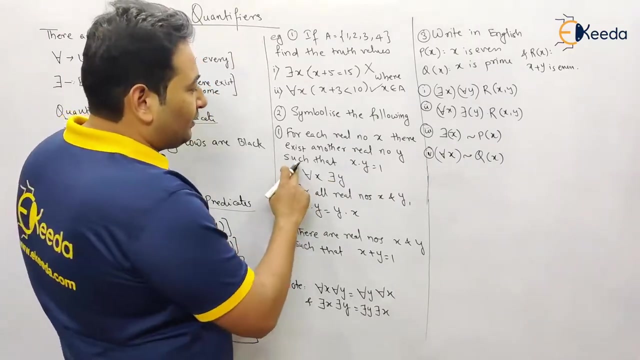 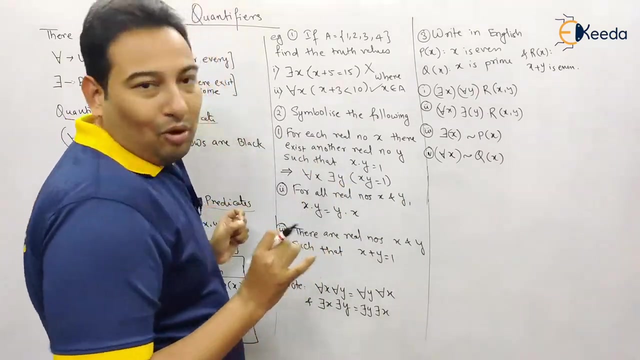 problem is in terms of x and y, both. so let's check. we need to write it down in the symbolic form. for each real number x, see, for each real number x, that means for all x, there exists real number y, there exists real number y, such that x, y is equal to one. see, you just need to read the things and write it on properly. it's. 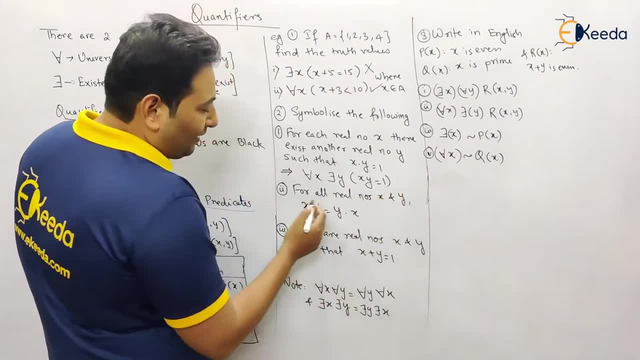 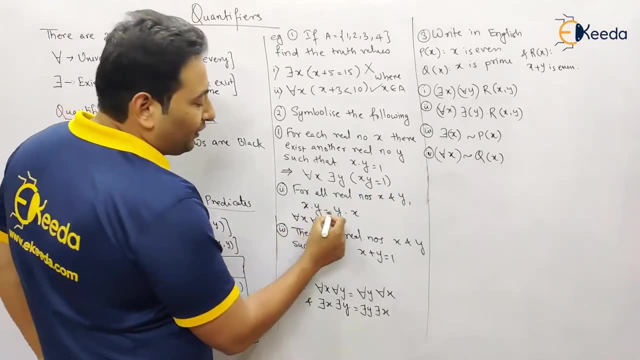 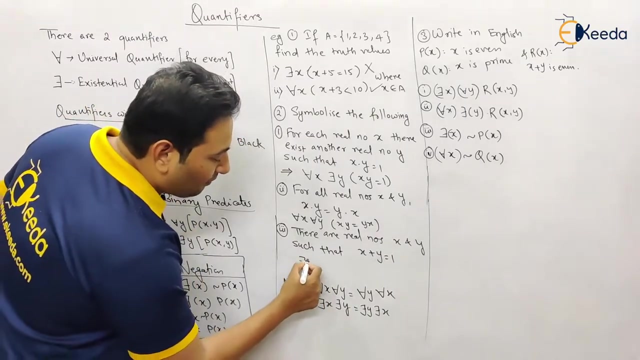 very simple topic: for all real number x and y, that means all x and y, all real numbers x and y. so that means: for every x, for every y, x, y is equal to y, x. what next? there are real numbers x and y. that means there are few real numbers x, as well as there are few real numbers y, such that 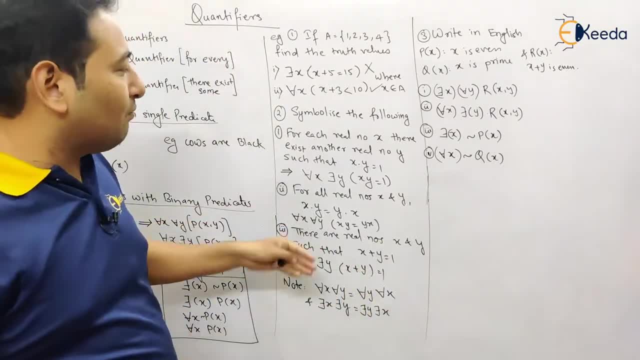 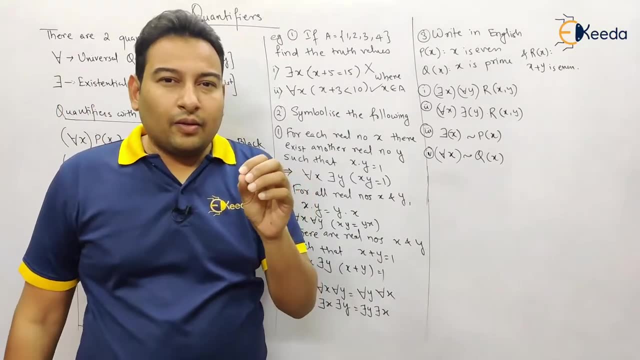 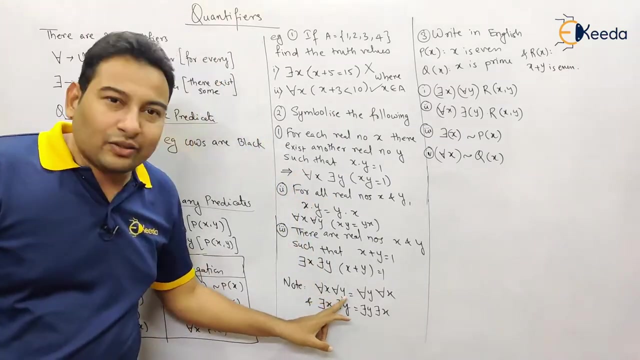 x plus y is equal to 1. so this is the way we can write it on these symbols from the given statement. a very important note here: if you have both universal quantifier or existential quantifier, you can swap their position. that means for every x, for every y, you can write it on s for every y, for. 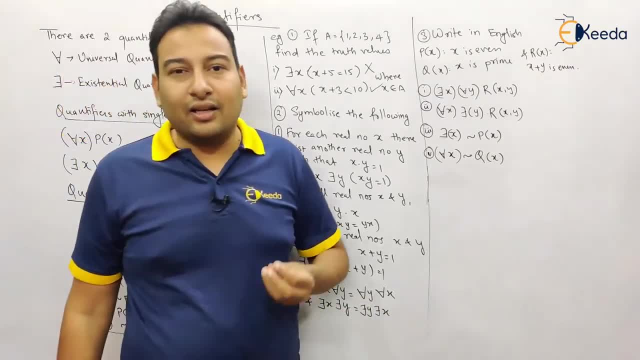 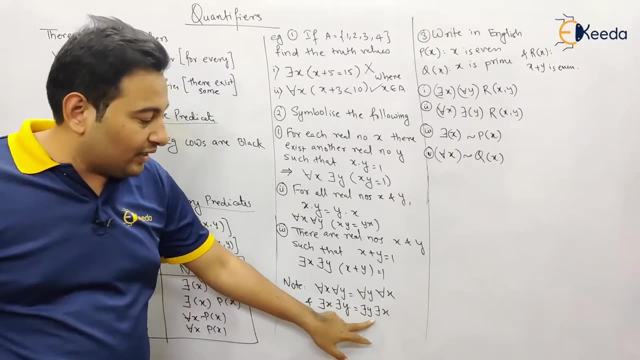 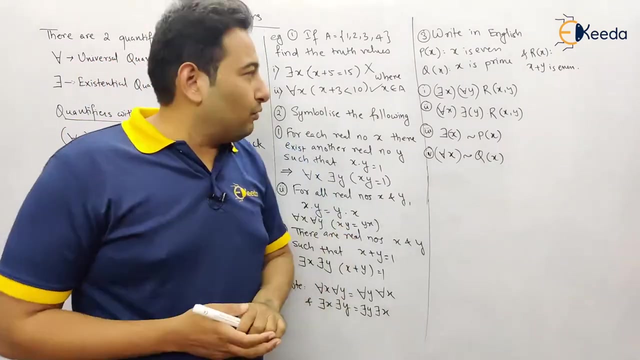 every x, so doesn't matter. and the same way it goes with the extension existential quantifier. there exists some x, there exists some y. you can again swap and write on this: there exists some y, there exists some x, so that is perfectly fine. but if you have mixed for a universal and existential quantifier, you cannot swap. for example, 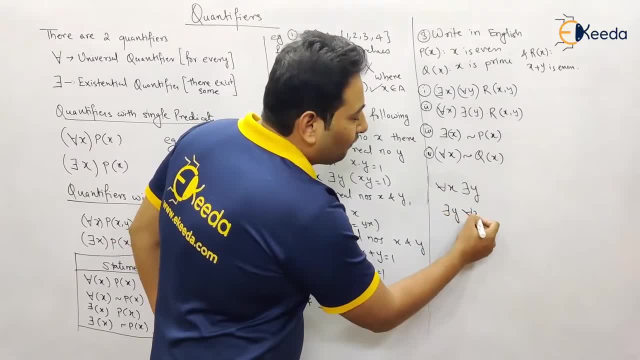 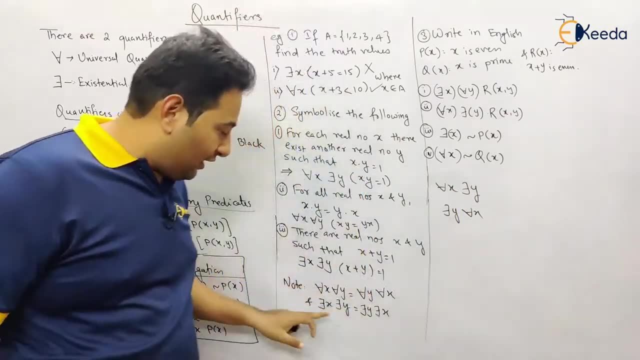 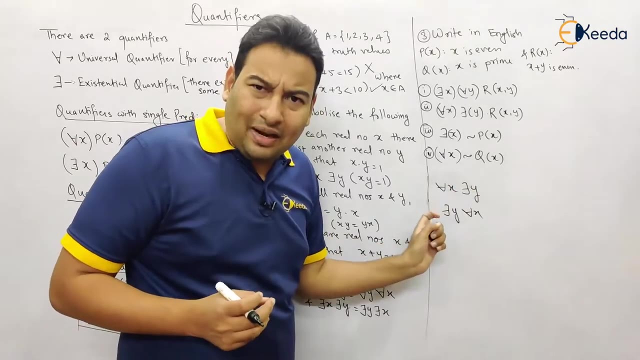 if you have something like this- you cannot write it down this way- you cannot swap their position, you cannot change their position. if both are universal, you can change. see here: if both are existential, you can change. but if one is existential and one is universal, order doesn't matter, you cannot change the order. is this clear? so this, this note you need to. 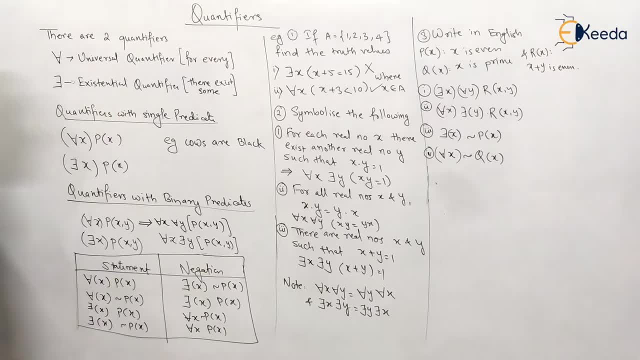 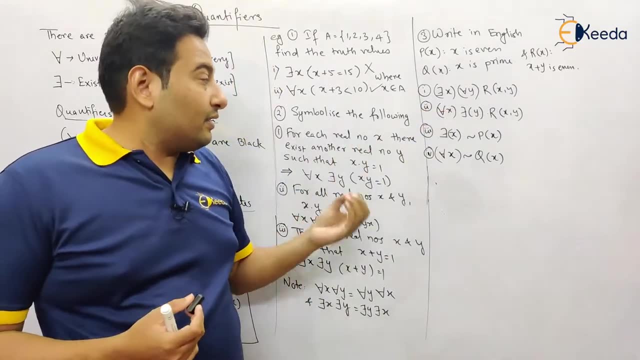 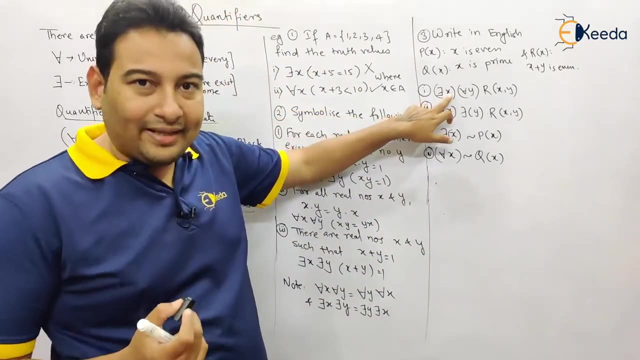 remember: let us move on and let us write it down. the last problem: write in english. so statements are given and we need to write it down. uh, the symbols are given, we need to write it down in the english statement. see, what does this mean for every? uh, sorry, there exists some x. for every y, r of x, y. 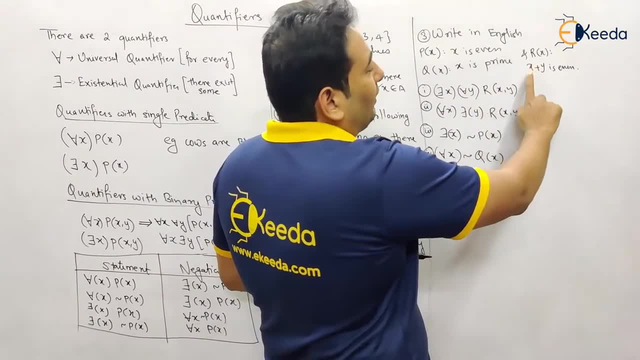 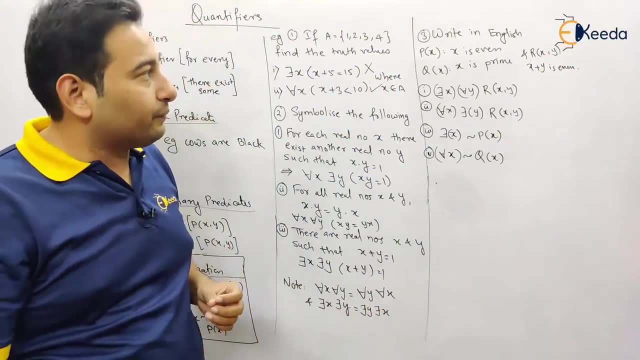 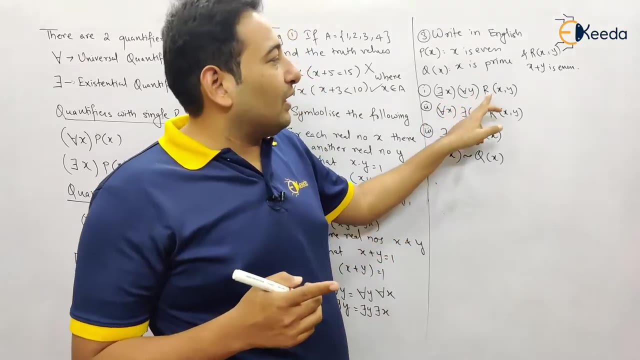 that means r of x comma y is what r of x comma y is. x plus y is even. so how? what will be the english statement of the sentence? there exists some x for every y. r of x comma y is true. that means x plus y is even that means. 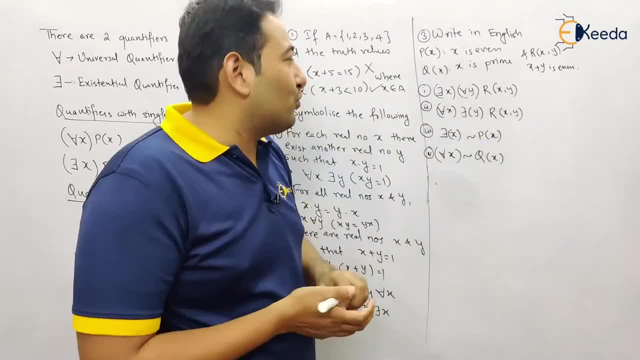 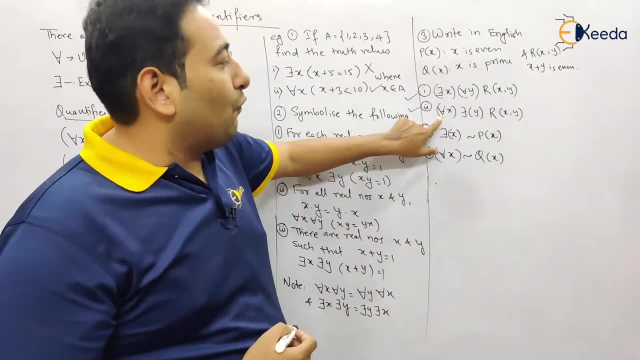 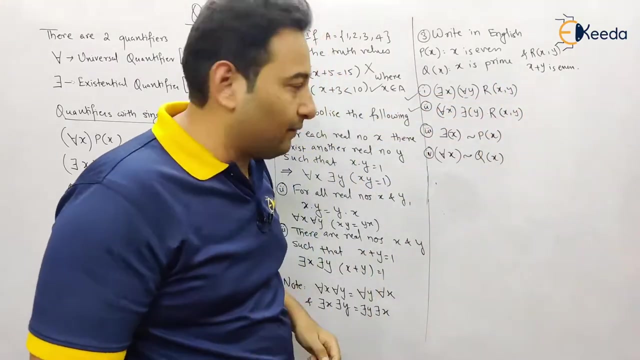 there exists some x for every y. x plus y is even so. this is this english statement for the first symbol. next, let's talk about the number two. for every x, there exists some y for which x plus y is even so. this is the next statement. next, there exists some x for which px is not true. what is px? 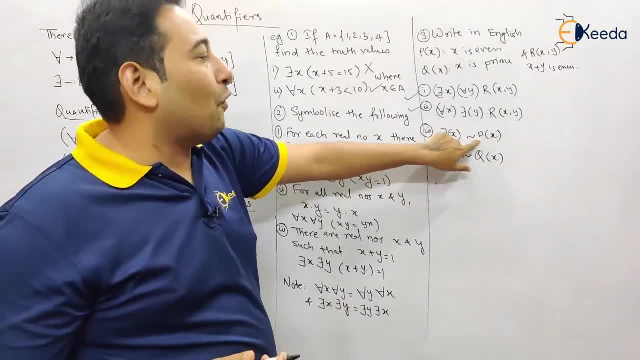 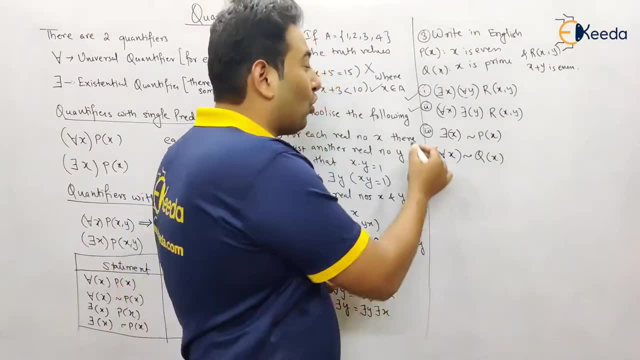 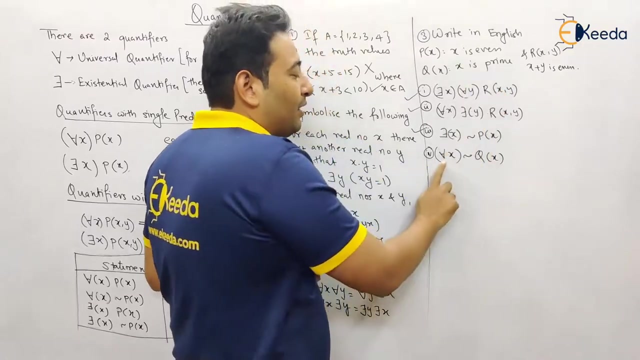 x is even. that means there exists some x for which px is x is even so opposite of that. so there exists some x for which px is odd. so this is the third statement. and finally, for every x, q, x is not true. x is prime. so for every x, x is not a prime number. so this is the way how to read, and 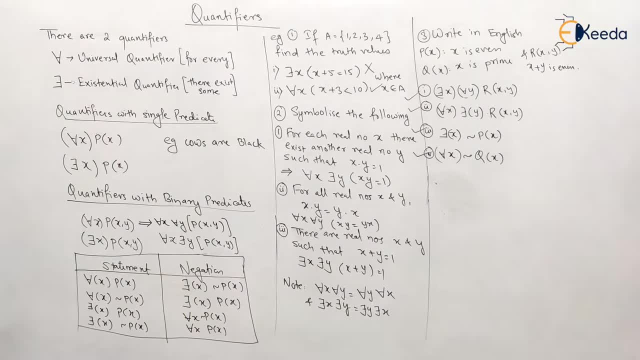 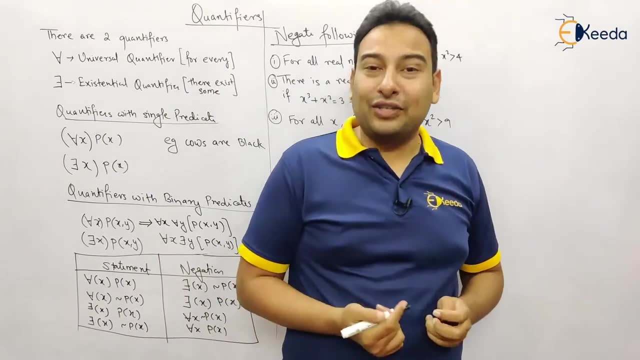 write it down, the quantifiers. now we'll discuss about negation. we'll see some example on negation. three statements are given and we need to negate it. we need to find its negation. the rules for negations are already- we have already discussed this. now, based on this rule, 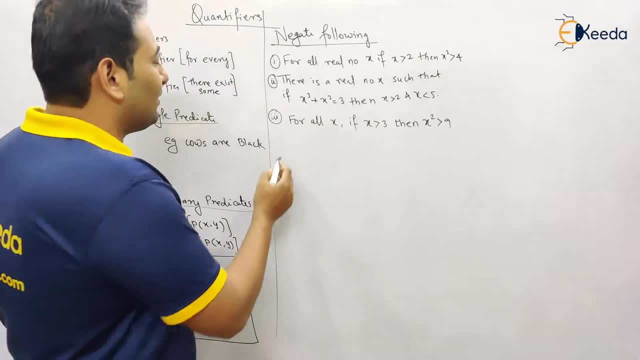 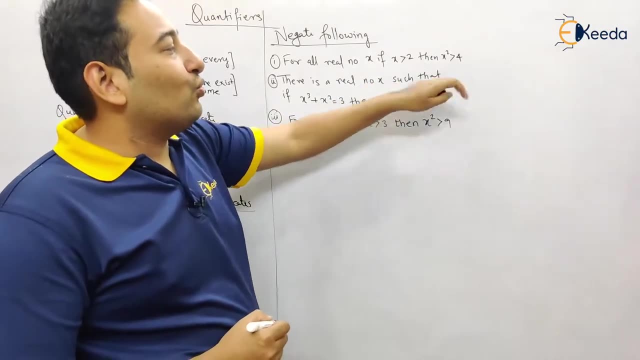 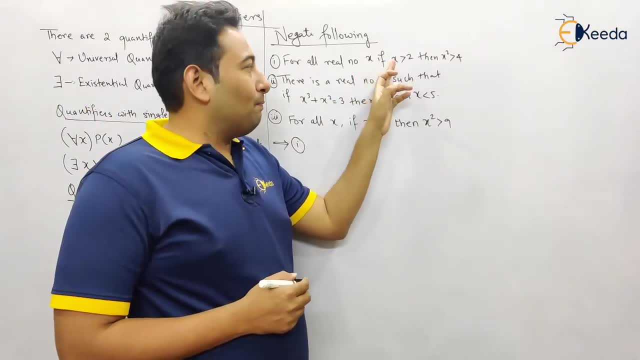 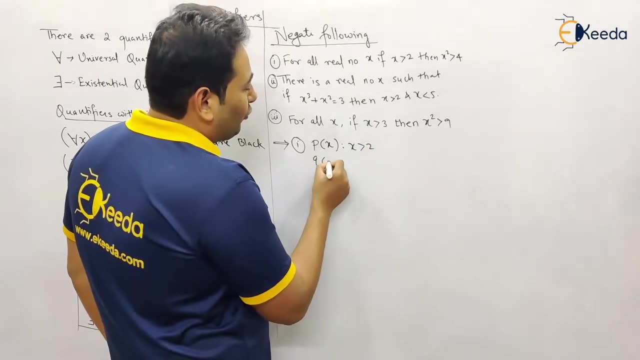 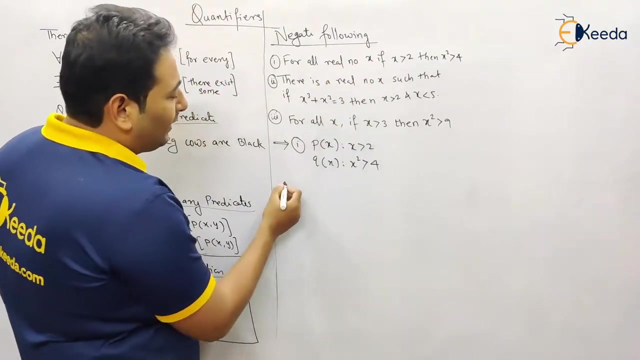 So let us start. Let us assume p of x is x is greater than 2. this is the assumption: p of x is x greater than 2 and let's say q of x is x square greater than 4.. Now for all real number x. that means for every x, what is given if x greater than 2? that means: 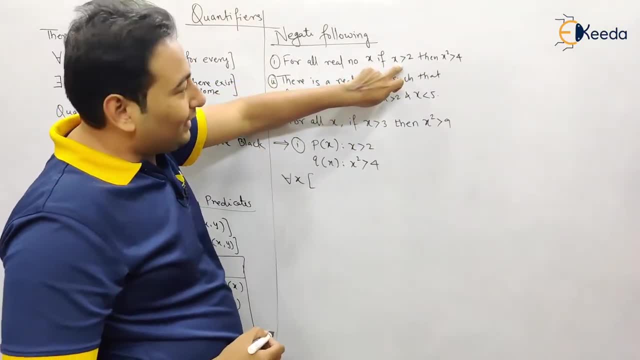 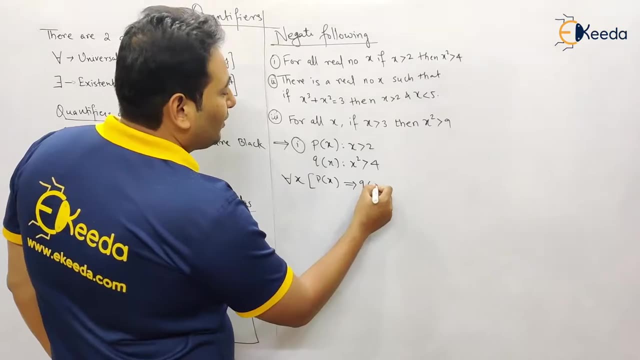 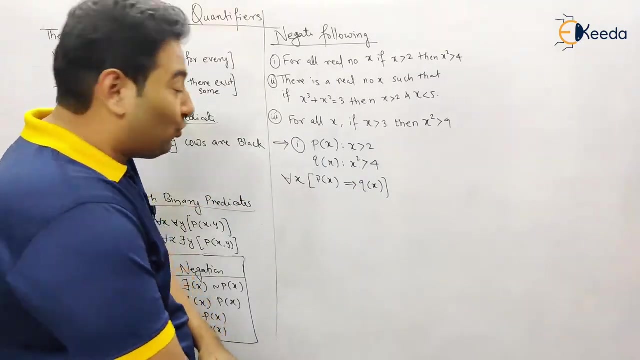 implies for every x. if x greater than 2, then x square is greater than 4. that means p x implies q x. So this is the statement meaning for every x. if x is greater than 2, then x square is greater than 4.. 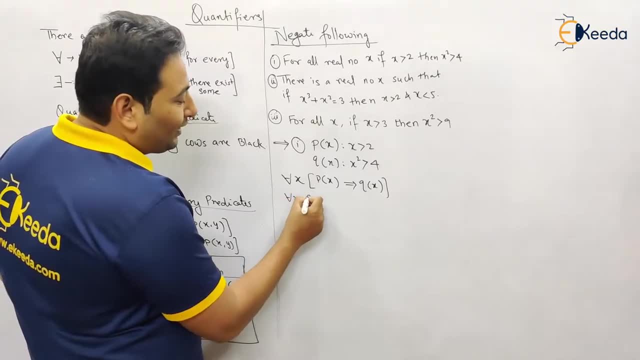 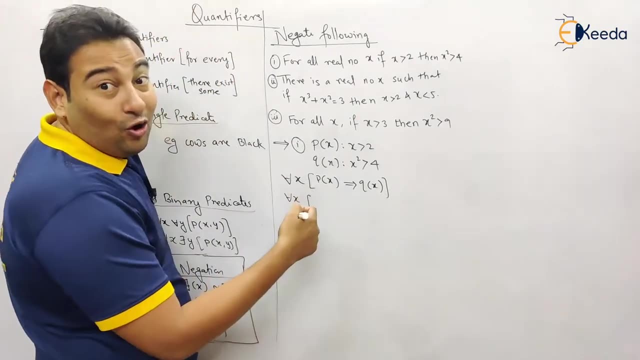 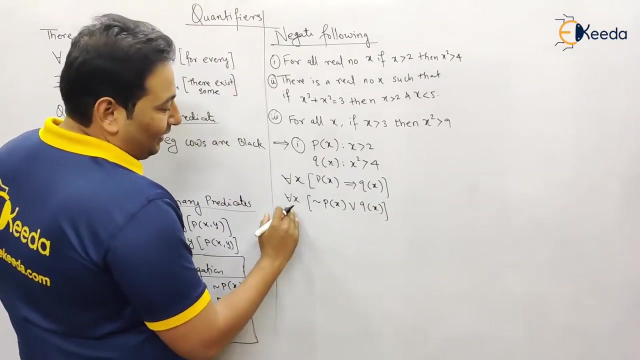 We need to negate it. So how to take negation. first of all, for taking the negation, Let us simplify this. what do you mean by this implication? negation p or q, negation of the first term or second term? Let's take this. let's take the negation of the end. see, this is what the required statement. 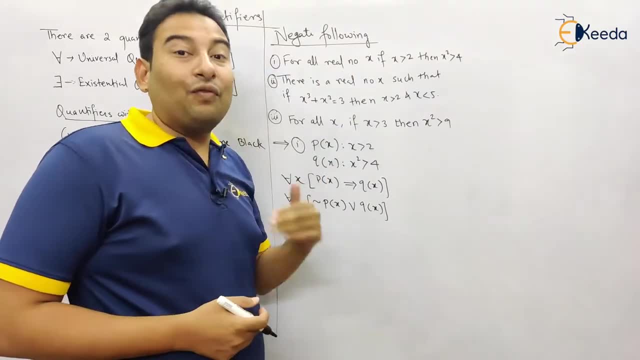 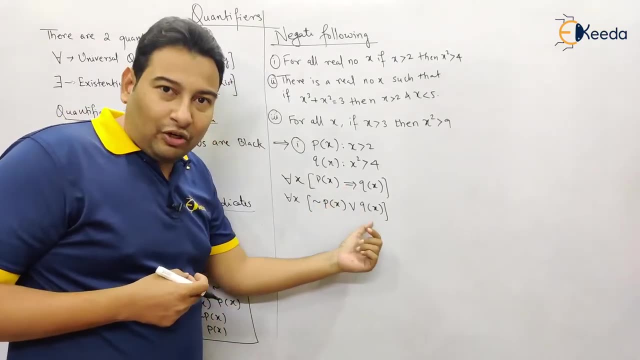 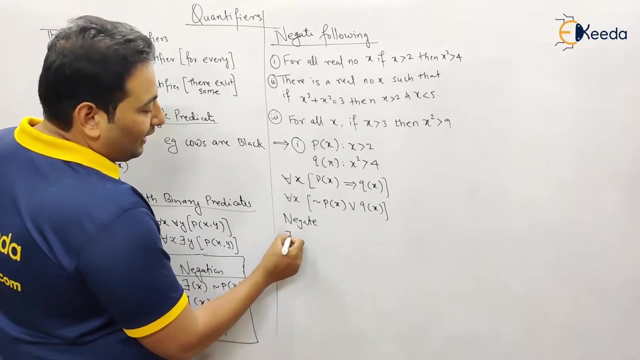 is: we just converted this into symbolic form. Now we need to negate it. we have not negated it yet. we just replace this implication with this particular property. Now we need to negate it. If I'll take its negation, then for every x becomes there exists some x and negation. 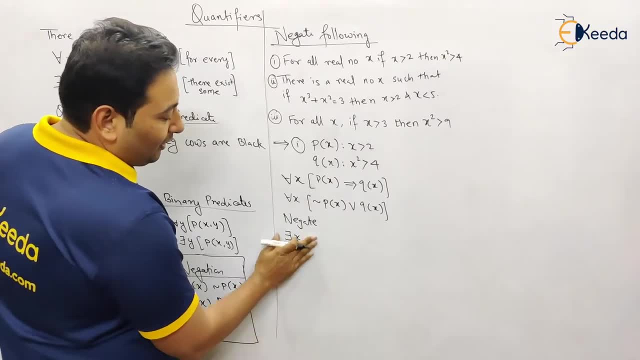 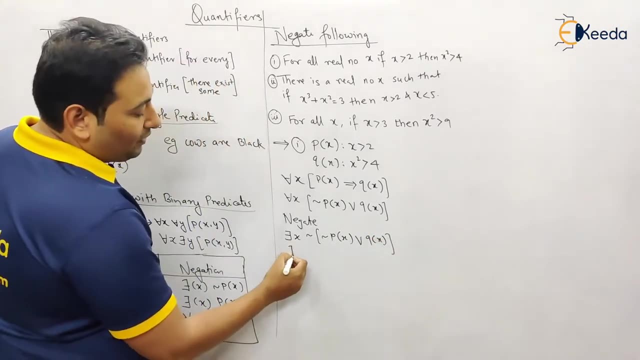 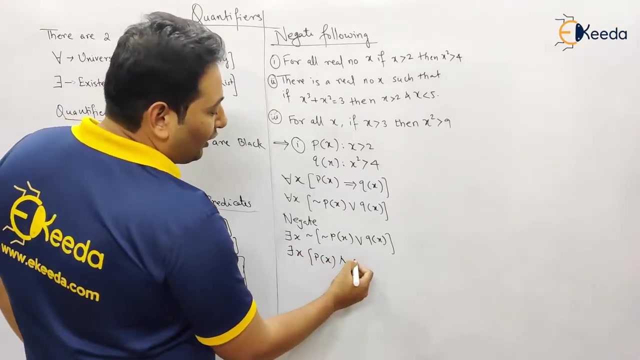 of this particular statement. So here there will be a negation. basically, If I'll open this bracket, this will be negation of x, this will be cancelled. So, in short, we'll get p, x, this or will become and- and this is what negation- of q, x. 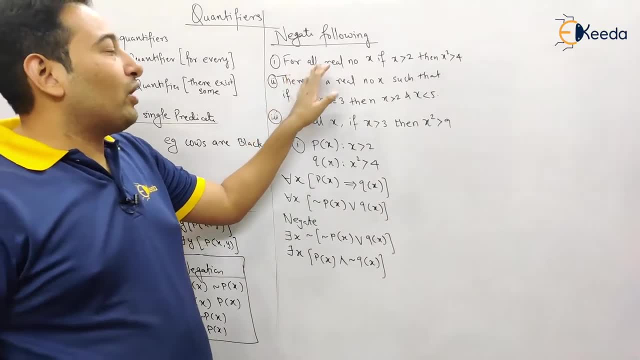 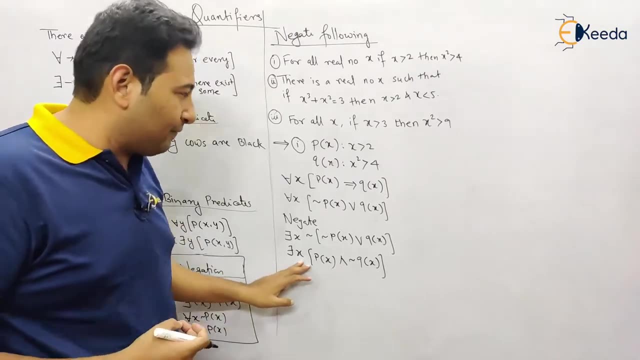 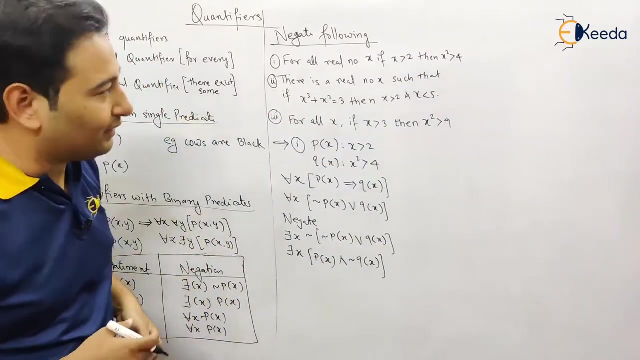 Now let us translate in English: It was for 4.5.. Now let us translate in English: It was for all real number x. So here there are. there are few real numbers, or there exists some real number x, for which x is greater than 2 and x square is not greater than 4.. 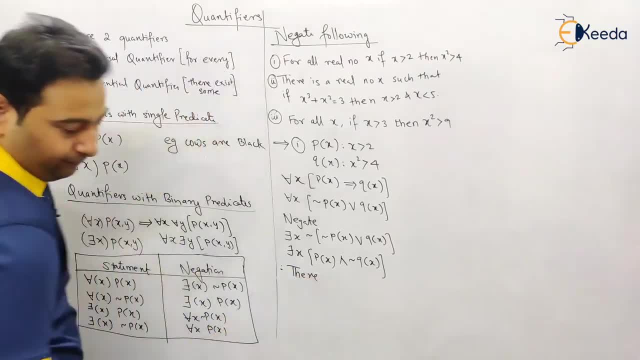 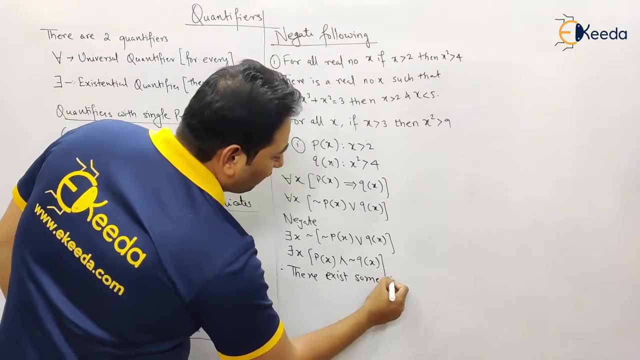 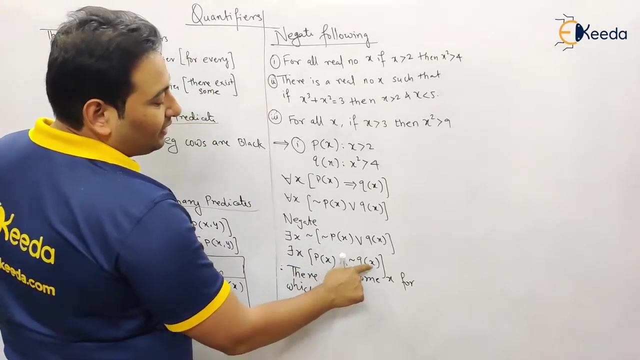 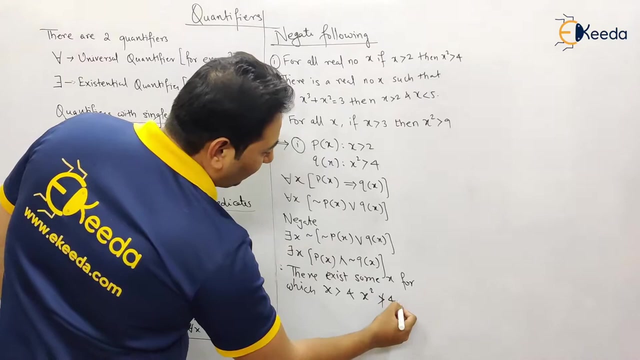 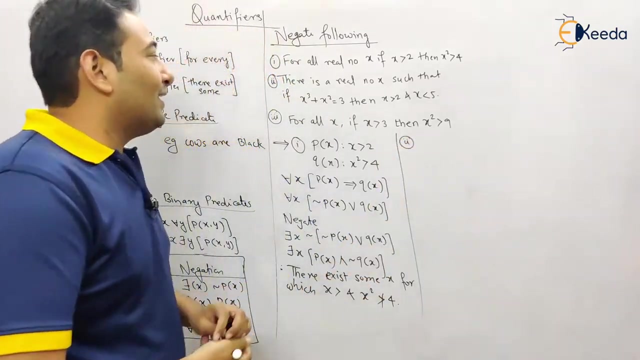 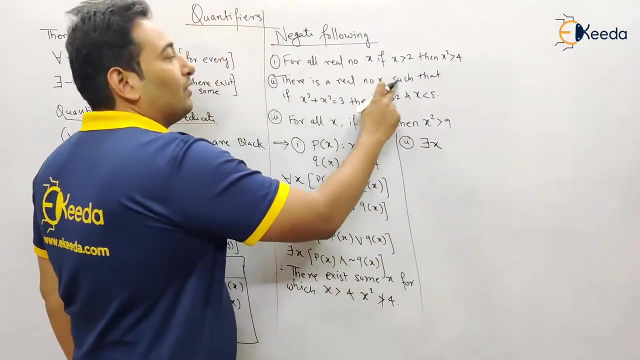 So the statement is: there exists some x for which. So this is your statement: negation of this particular statement. let's talk about the next statement, statement number two: there is a real number x. there is a real number x. that means there exists a real number x such that if x cube plus x square is equal. 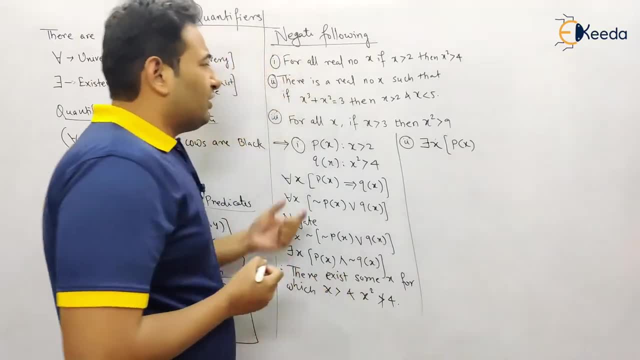 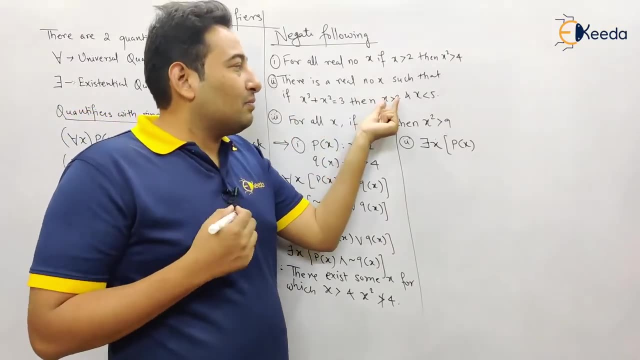 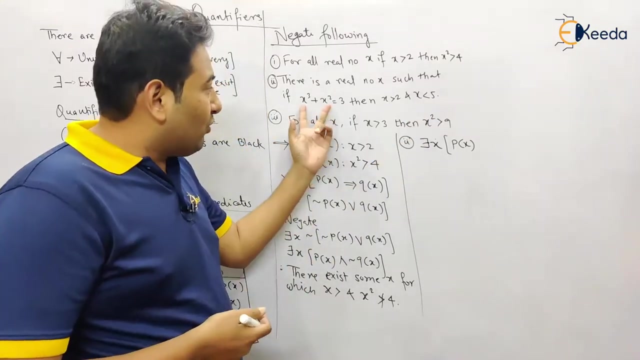 to 3.. Let me assume this is p x. obviously you have to write it down like this in the exam: let. so I'm assuming this is my p x, this is my q x and let's say r x. you have to assume this. you have to show this in the exam. let p x is equal to x. cube plus x square is equal. 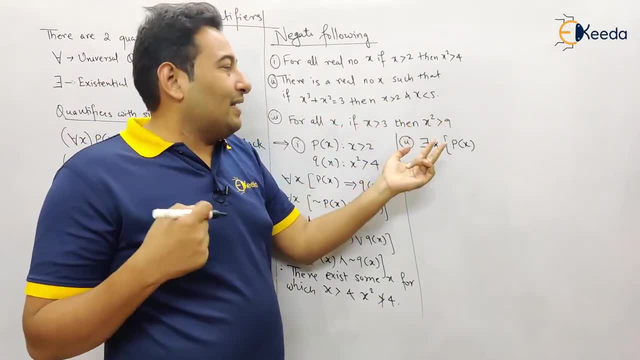 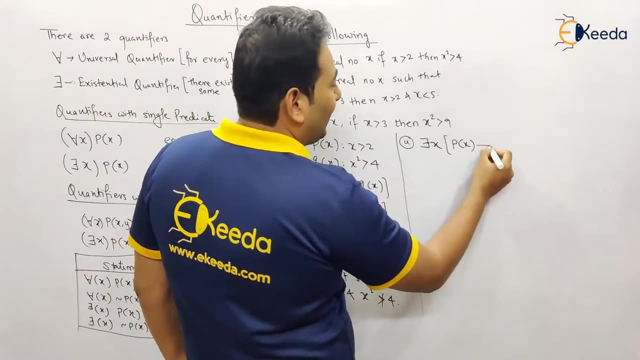 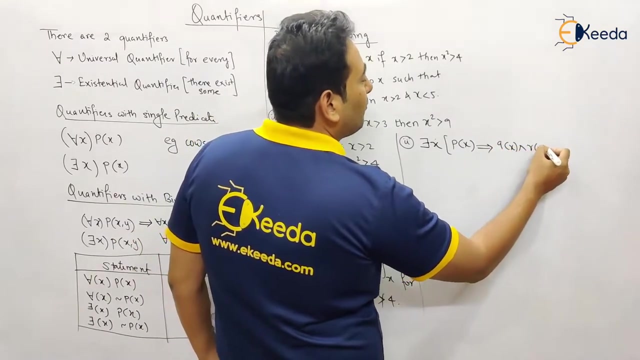 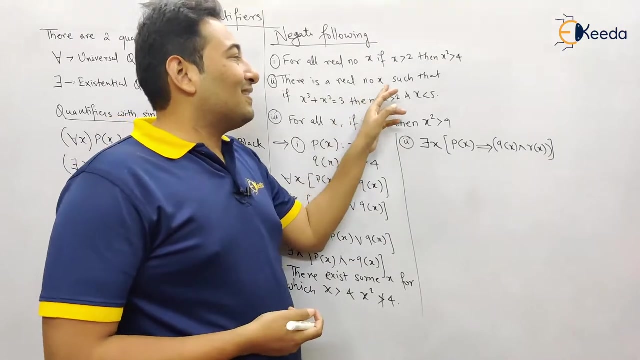 to 3, q x is equal to x is greater than 2 and r x is x is less than 5, if there is a real number, x, such that, if this is true, Then Okay, This and this, so q x and r x. so this is your symbolic form. there exists some x such that: 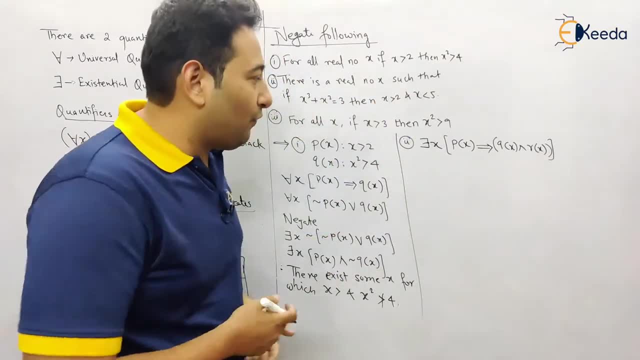 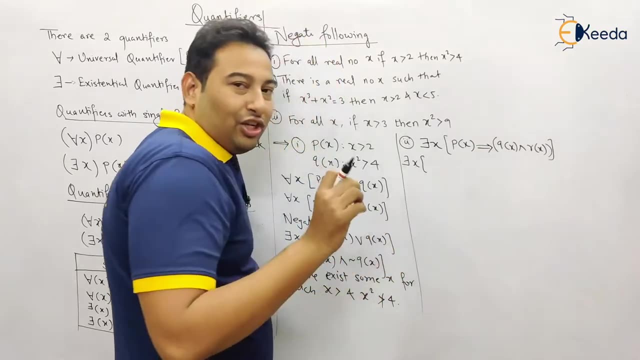 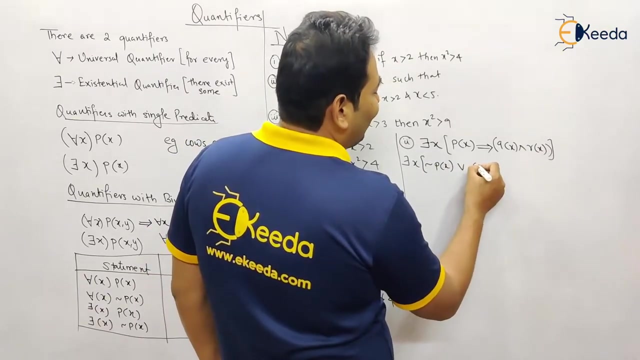 if this is true, then this and this. so, first of all, before taking negation, let us simplify. first of all, let's convert this implication into negation p or q formula, so negation of the first term, or q that is second term. so q, x and r x. 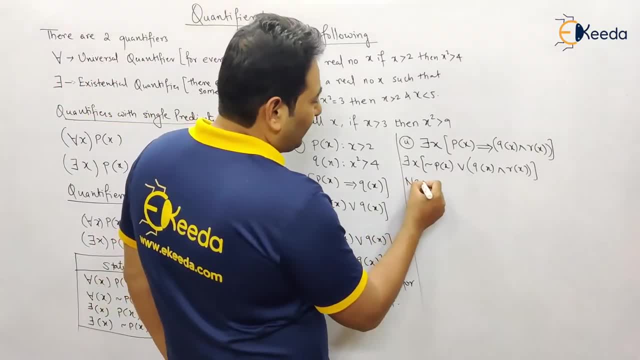 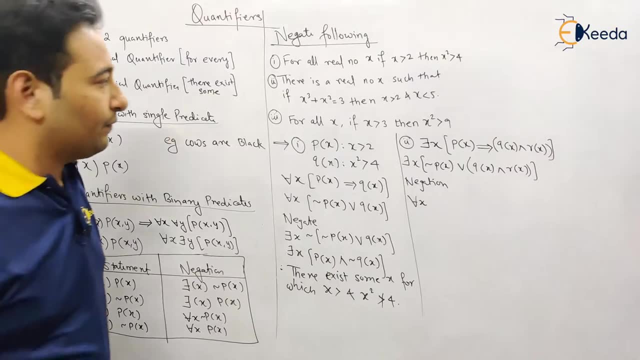 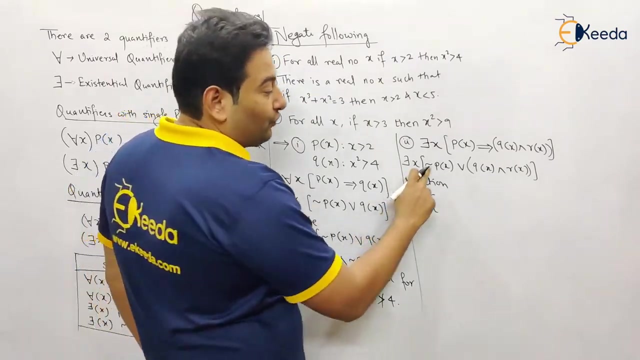 What next? now we're going to take its negation. so if I'll take its negation, there exists some x will become for every x. Now I'm directly taking the negation, so this will become p? x, because negation, negation will cancel each other. 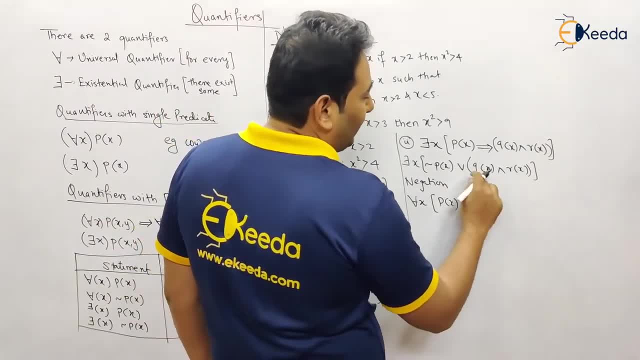 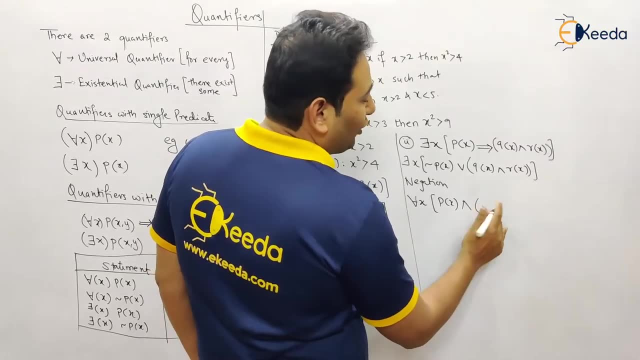 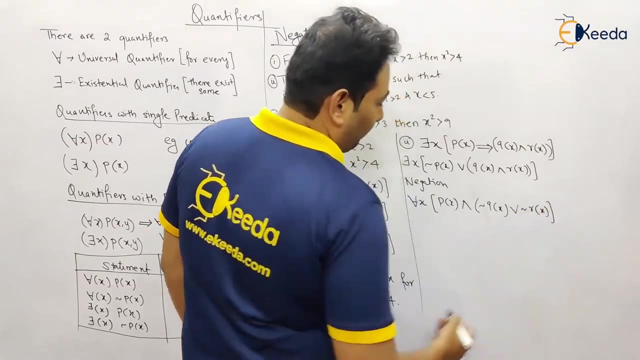 So this is p x, this and or will become and and negation of this particular term. so if I'll take negation and if I open the bracket, so this will become q x negation of q x. This and will become or and this will become negation of r x. 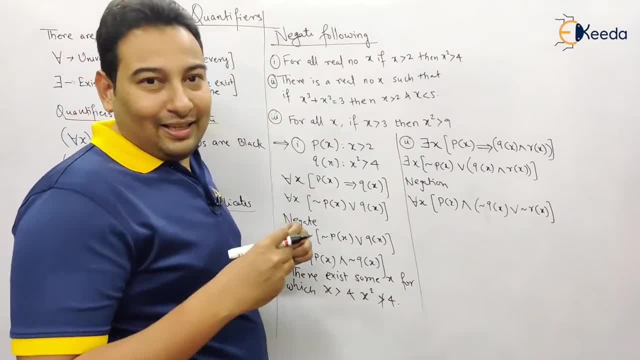 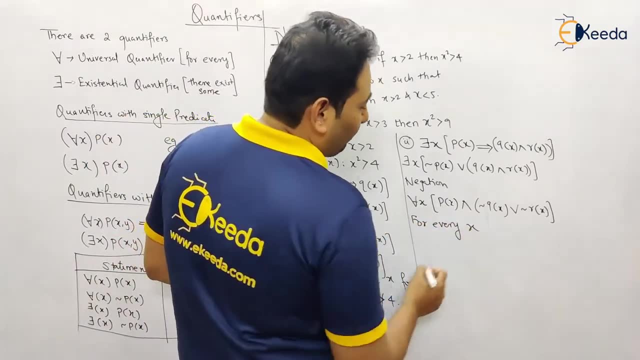 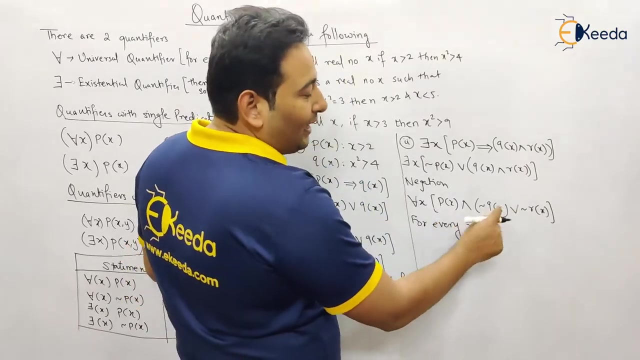 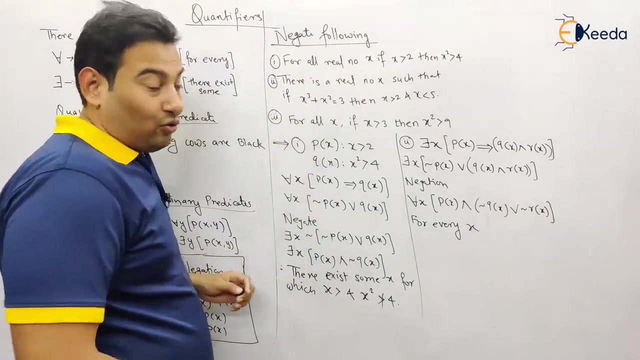 So this is your negation form. now let us write it on in English sentence: so this means: for every x, p of x, and so p of x is true, and either this q of x is not true or r of x is not true. so this is the meaning. so let me read it again see. what does this statement means? for every. 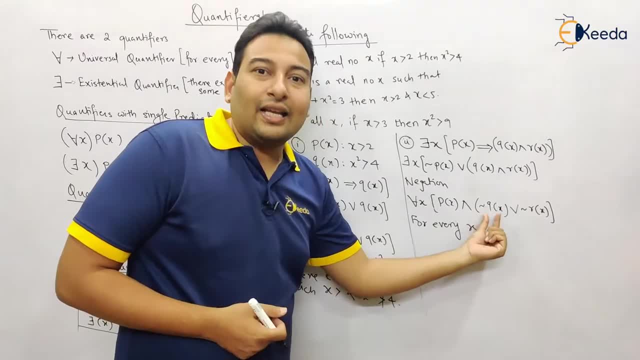 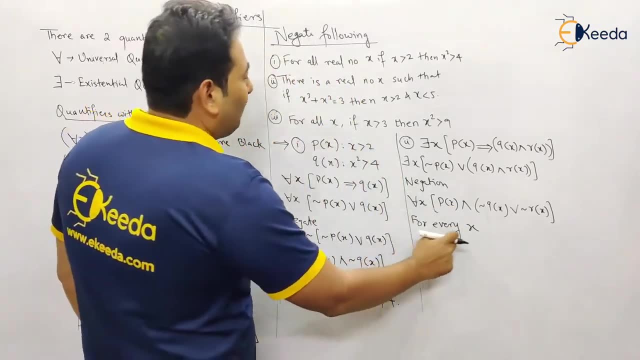 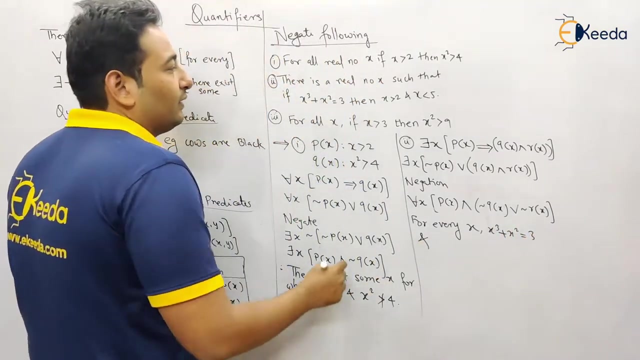 x, p x is true, and either this is not true or this is not true. so this is the meaning of the statement. so p? x is true is what: For every x, x, q of x, p, of x, Multihutil plus x, square is equal to 3 and 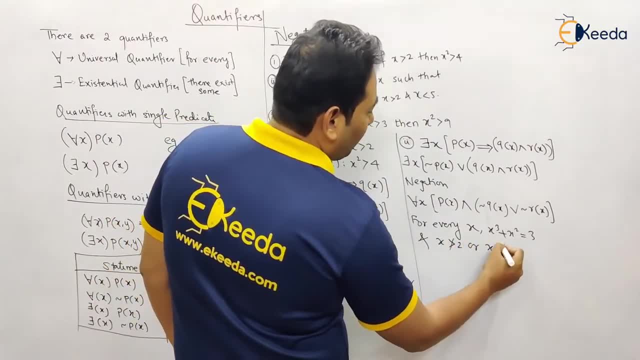 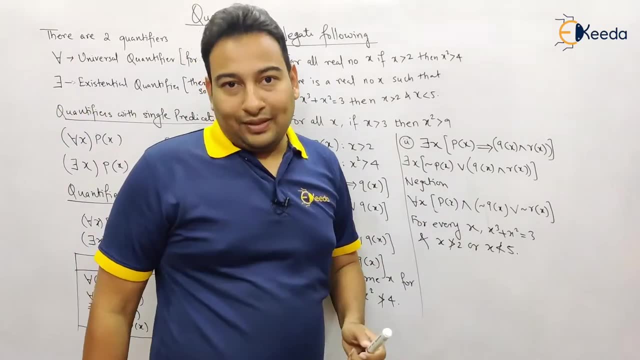 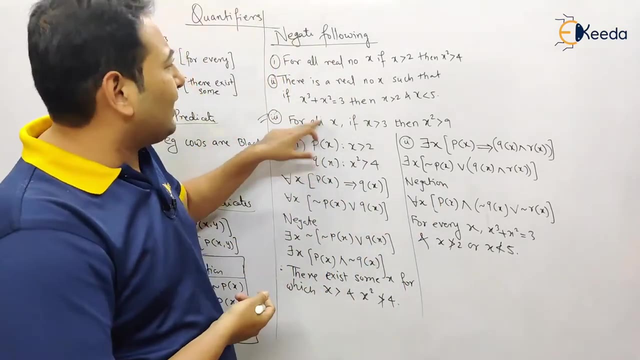 x is not greater than 2 or x is not less than 5.. So this is the English statement of this particular symbolic form. is this clear? Now suppose you find something like this. Now see third example you going to solve by yourself: exactly similar to problem of. 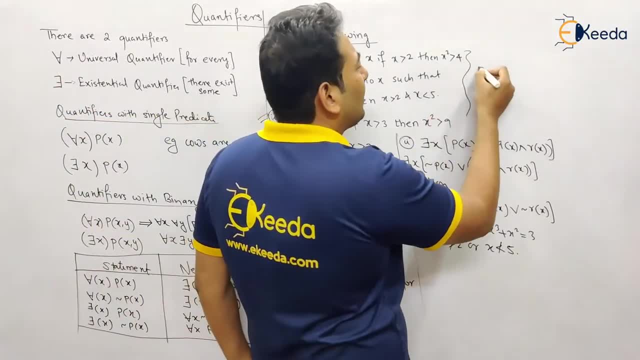 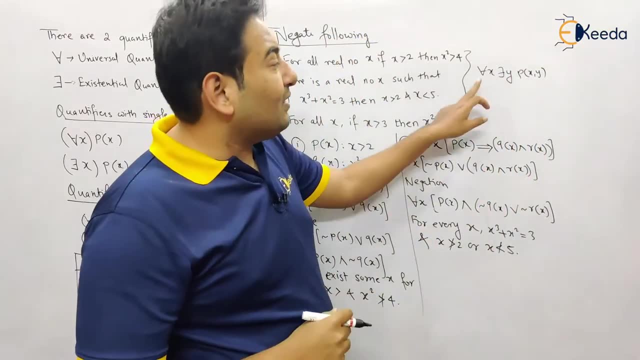 1. So this is your home work problem, and suppose you have something like this. let me say: for every x exists some y, p of x comma y. now what does this statement mean? this means for every x there exists some y, for which p of x comma y is true. and if i want to find this negation, so this will, this will. 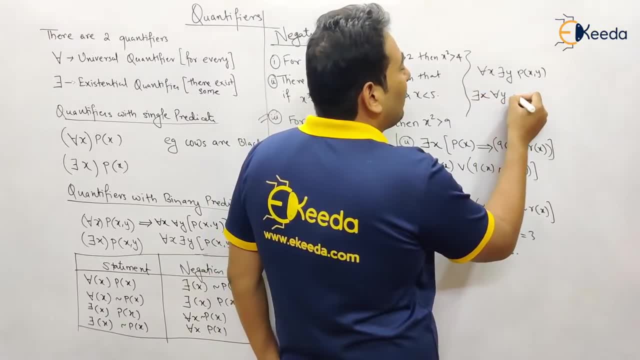 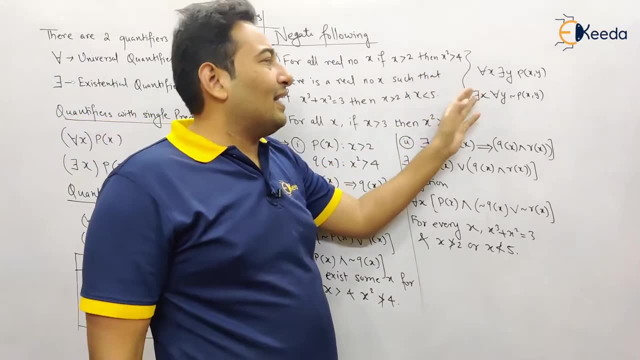 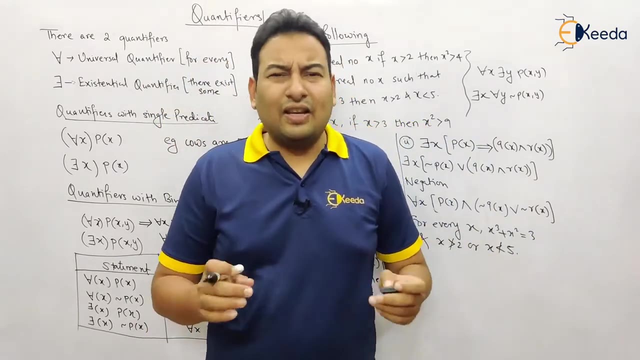 become. there exists some x for every y. p of x comma y is not true. so if there are both universal and existential quantifier, you have to take negation accordingly. so that's it all about quantifier. it's a very simple video and important topic also. hope you understood. we're done with it. thank you for watching this video. take care.